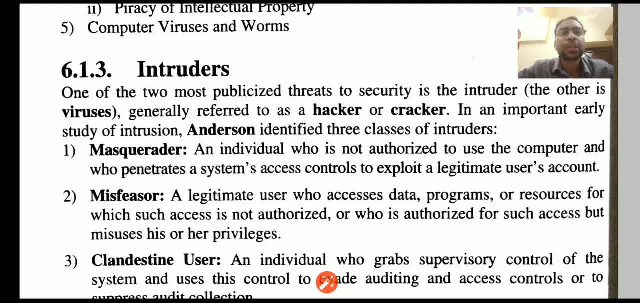 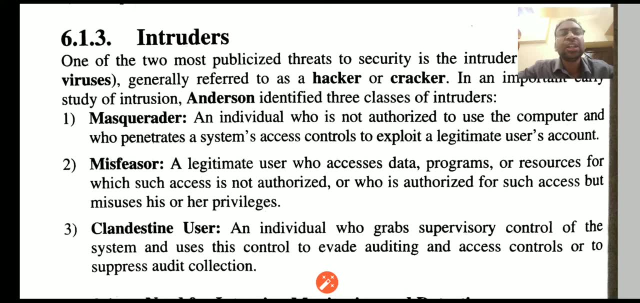 try to change the data, the security and other things in your systems and they try to harm the system. So the main intruders, the types of the intruders, if we will discuss there are three types of intruders depending upon the access they can gain on the system. The first are masqueraders. 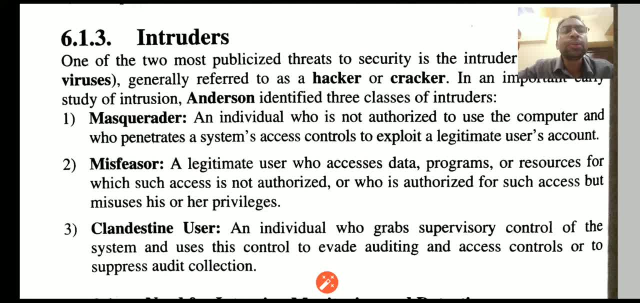 and individuals who is not authorized to use the computer and who penetrates the system's access controls to exploit beginner users account. So masqueraders are not basically the authorized users of the systems and they try to gain the access to the system. Then the next are misfeasors. So misfeasors basically are: 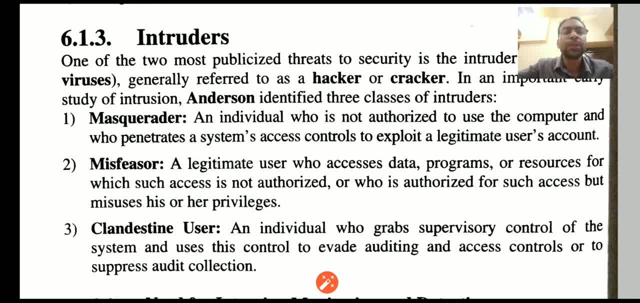 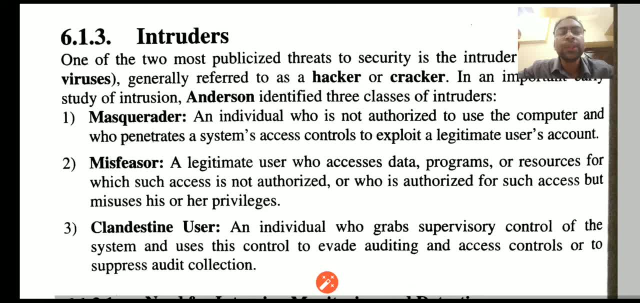 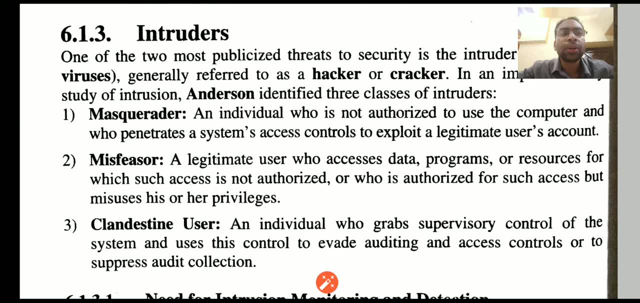 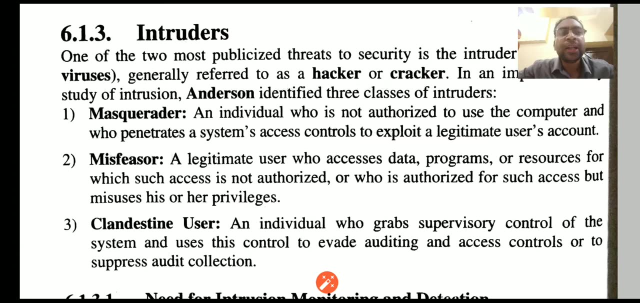 the authorized persons. They are legitimate users of the systems who have some access grants to access the data. So these are the legitimate users who access data, programs or resources in which in such a way that they are not authorized. So, basically, they are authorized to access another data and they try to access the data for which they are not authorized. So these 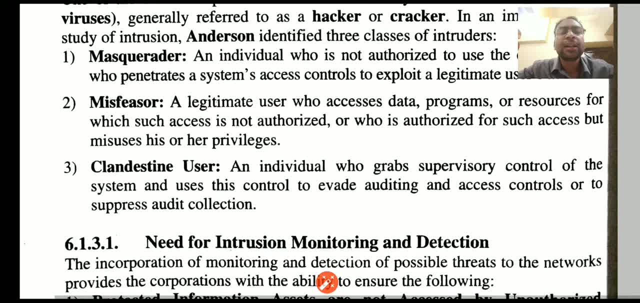 are misfeasors. And the third type, that is, clandestine users. They are the individuals who gains the supervisory control of the system, try to gain all the controls on the system, all the controls of the systems, and try to evade the auditing and other access controls to 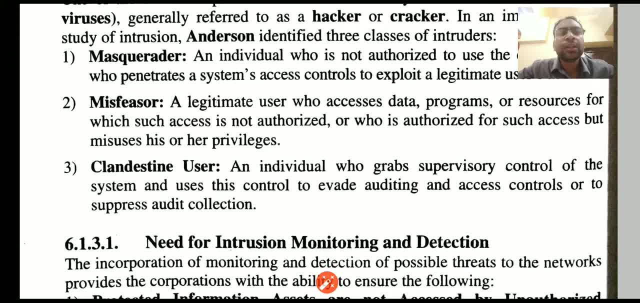 support the audit collection. So these are the three types of misfeasors, And the third type is the types of the intruders which can harm your system by gaining different types of access into the system. Now let's discuss what is the need for the intrusion detection and monitoring in your 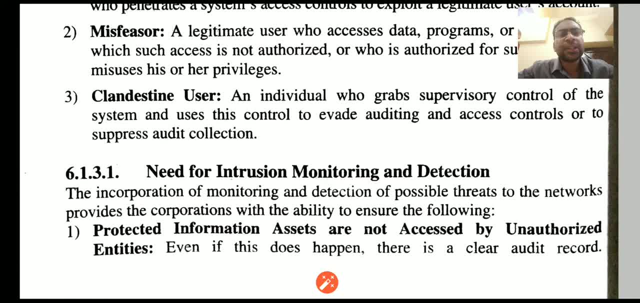 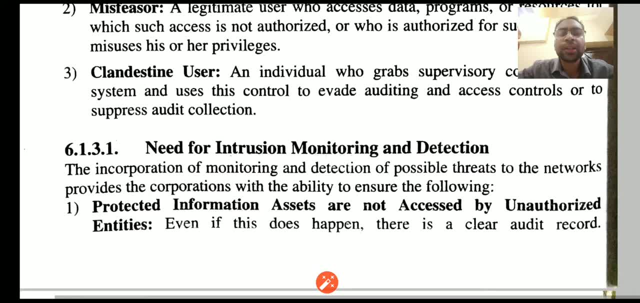 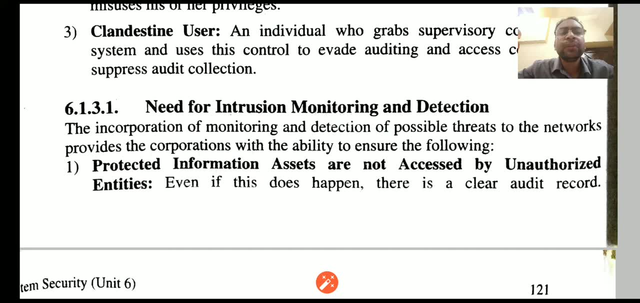 system. Obviously, any hacker, any cracker, any such individual who tries to access the data in unauthorized way must be monitored and must be detected so that we can prevent our system for such types of attacks. So the first we can see, the first need of intrusion monitoring is: protected information assets are not accessed. 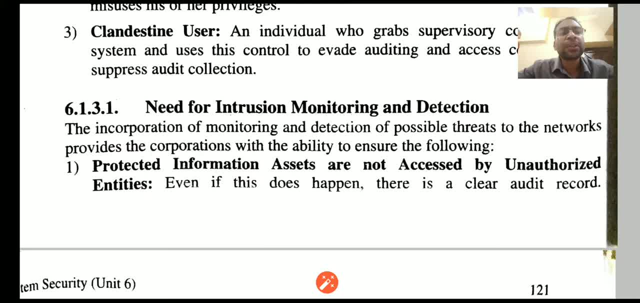 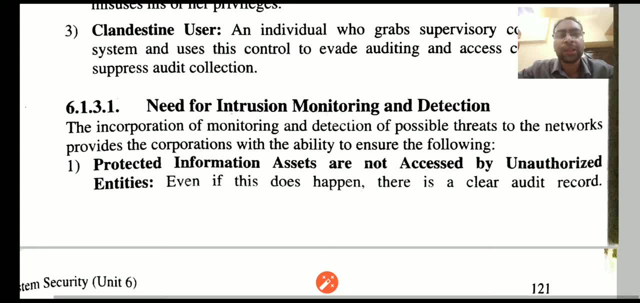 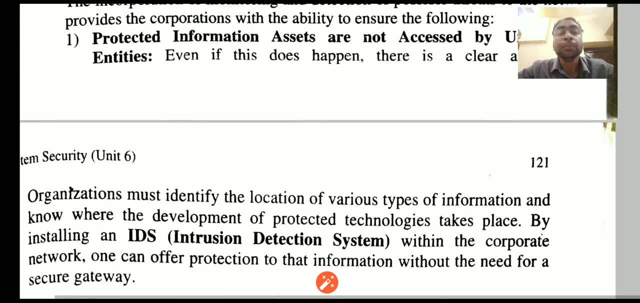 by unauthorized entities. Whatever the assets you have, whatever the data you have, if it is protected, then it must not be accessed by the unauthorized entities. So this can be monitored, and that is why we need the intrusion monitoring and detection system. The next need is the 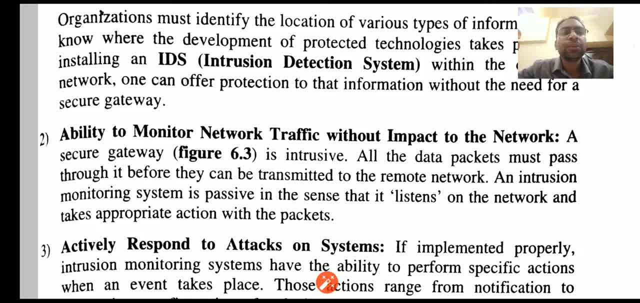 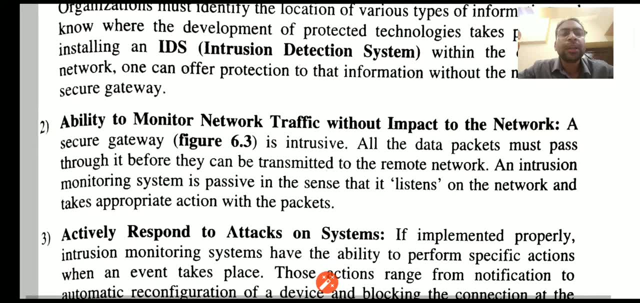 ability to monitor network traffic without impact to the network. So network traffic is an important thing. We had already seen the traffic analysis concept, where we analyze the traffic and, according to the analysis, we identify whether there are intruders on the network or not. So this will 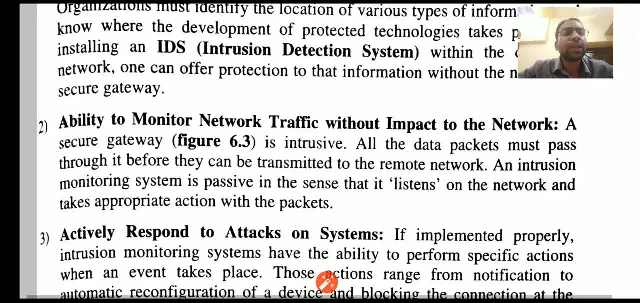 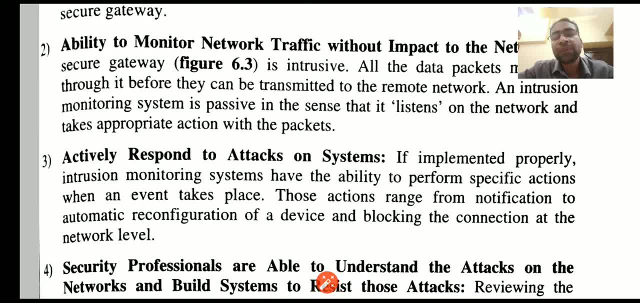 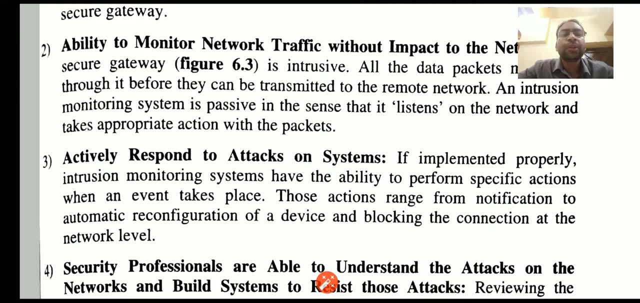 provide us the monitor, the ability to monitor the network traffic without impacting onto the network. The next reason is the actively respond to attacks on system. As soon as we'll detect an attack, as soon as we identify with the help of the monitoring, we can react. 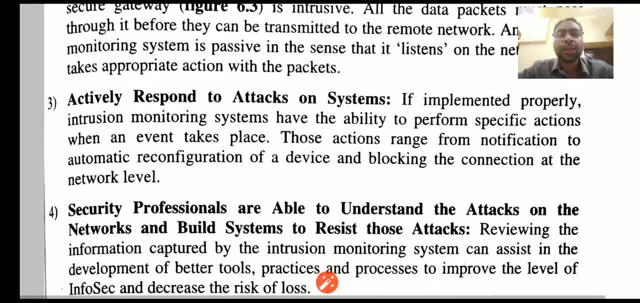 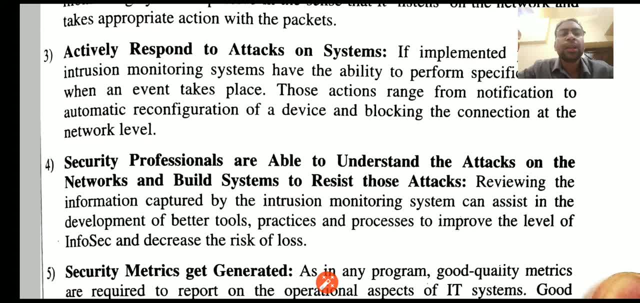 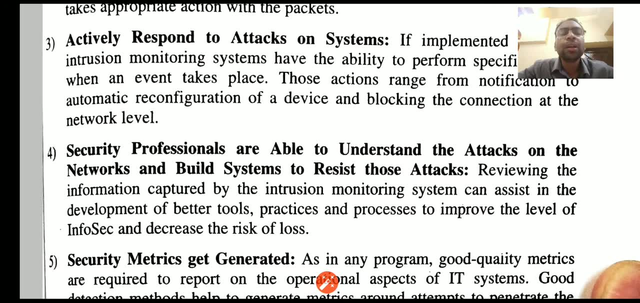 to the attack and perform the necessary actions. Security professionals are able to understand the attacks on the network and build system to resist those attacks. By the help of the monitoring and detection, we will be able to identify that from where the attacks can occur, what types of attacks can be occur And, depending upon these information, we can 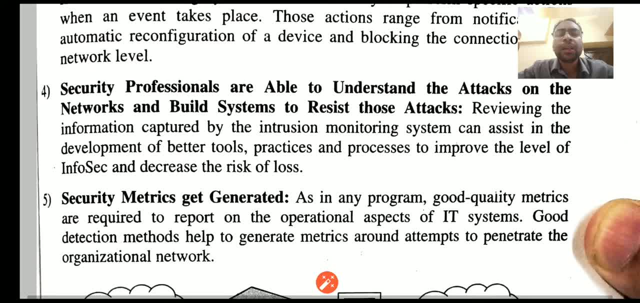 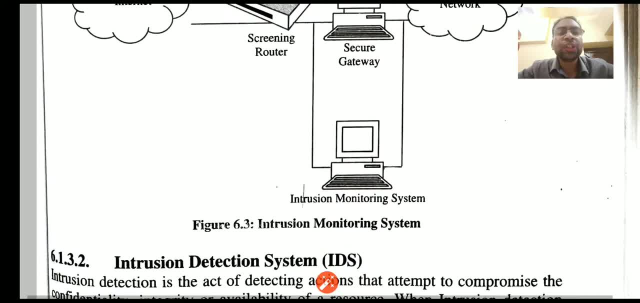 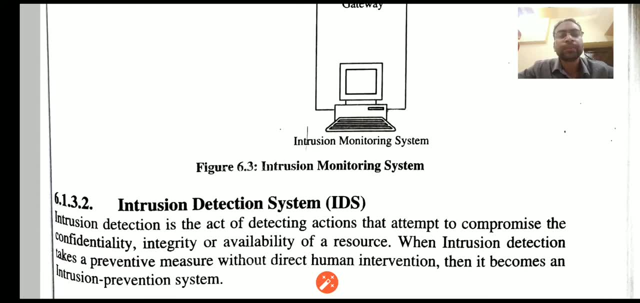 build the resistant systems, Security matrix get generated and depending upon these matrix, we can identify the potential of our security system. So for these purposes, intrusion detection system is required. Now, what is the intrusion detection system? Basically, it is a system that performs the 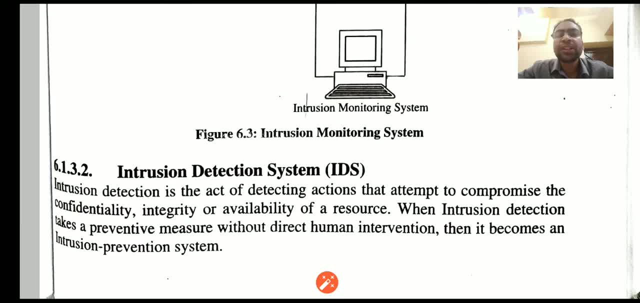 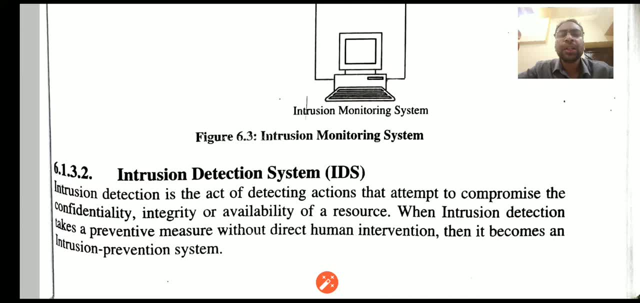 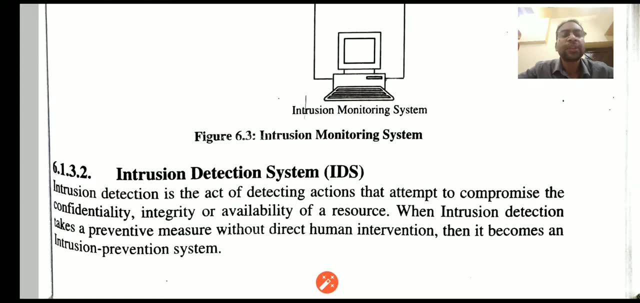 detecting actions that attempts to compromise the confidentiality, integrity and availability of a resource. So these are the three major definitions terms: confidentiality, integrity or availability. So we always protect these three terms in any network system, And IDS is a basically system that will detect such actions which are trying to compromise with these security. 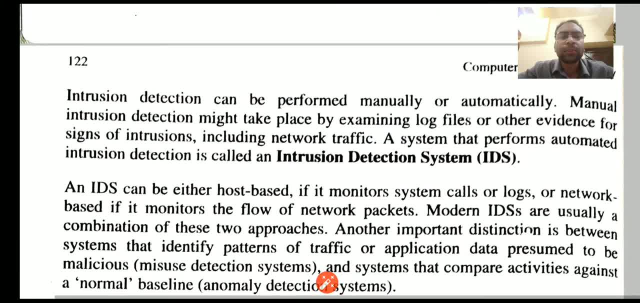 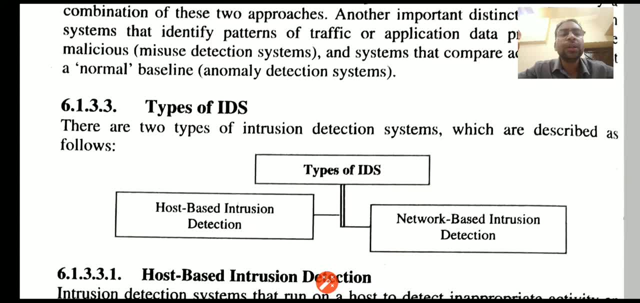 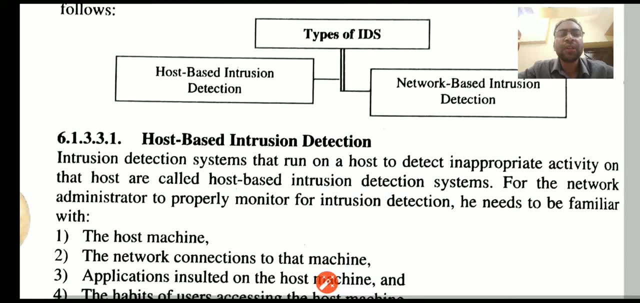 terms. Now let us talk about the types of IDS. So there are two types of IDS. One is the host based intrusion detection and another is the network based intrusion detection. So what are the host based, Where the intrusion detection system run on the host machine to detect? 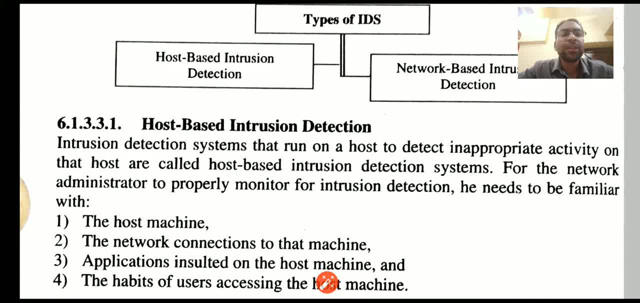 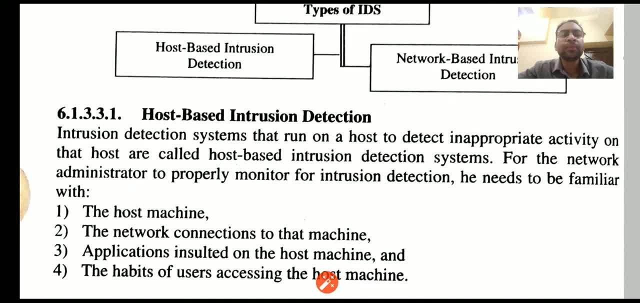 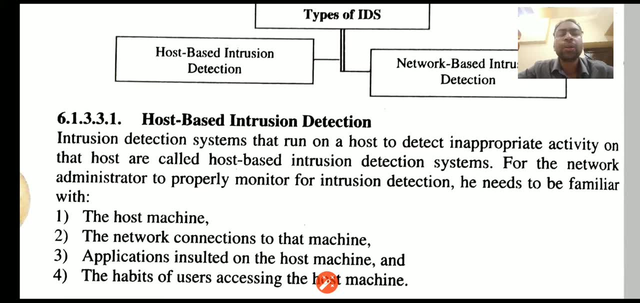 inappropriate activity on the host and these are called host based intrusion detection system. So they do not reside on the network, They do not monitor the network data. They reside on the host and perform their all monitoring and detection onto the host. For the purpose they must be familiar. 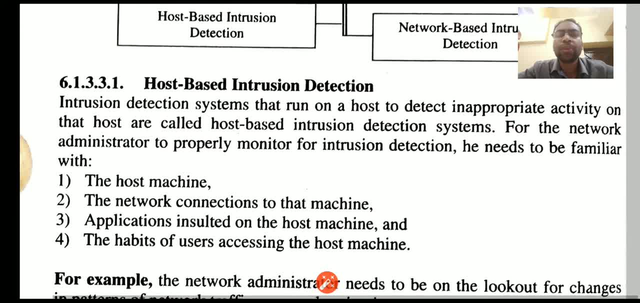 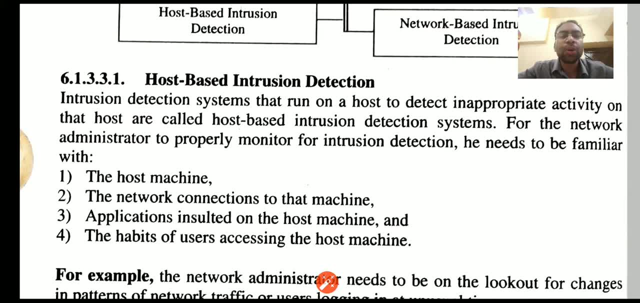 with these components, or we can say they must, it must have these components. The host machine should be there. The network connections to the machine should be there. Applications that is installed onto the host machine. host machine that will perform the monitoring and detection. 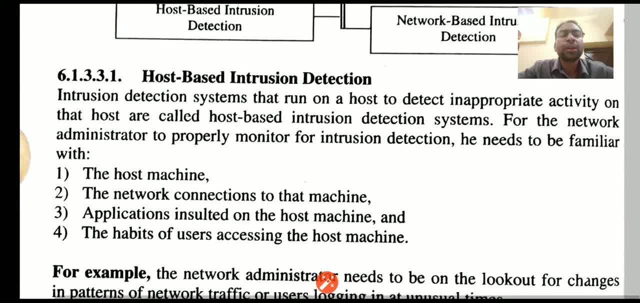 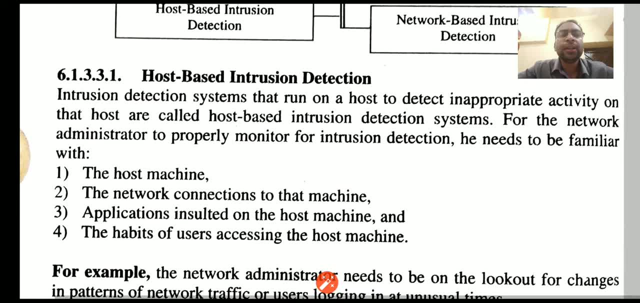 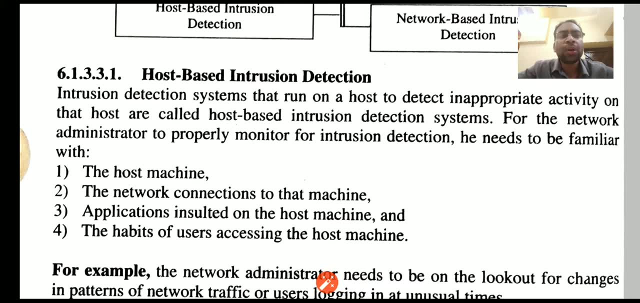 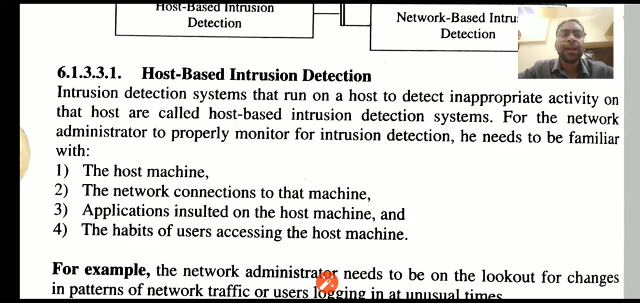 and the habits of the user who access the host machine. Obviously, the habits are required, because you can only identify the unauthorized access or unauthorized actions whenever you know who are authorized or how the authorized access is being performed. Then only you will be able to differentiate from a normal action and from an abnormal action. The next type is the 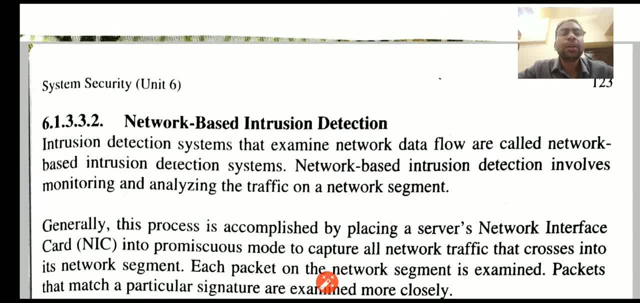 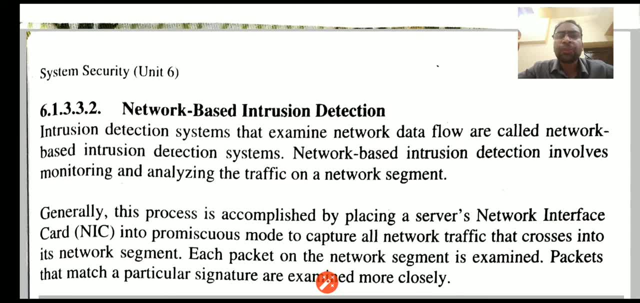 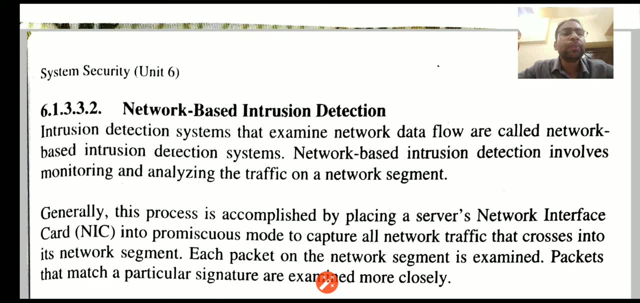 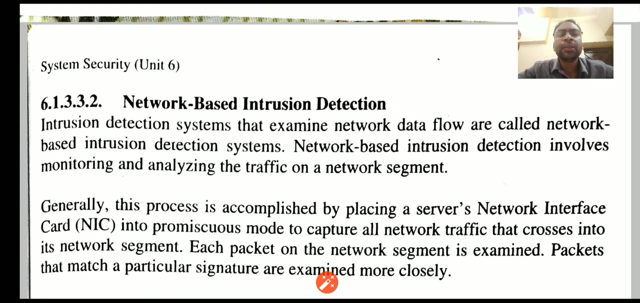 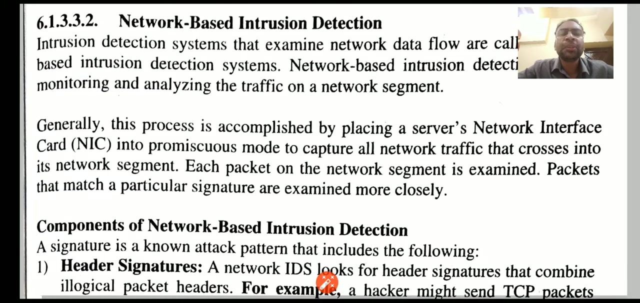 network based intrusion detection system where the network data flow is examined. Excuse me, the network data flow is examined and based on the intrusion detection network based systems that involve monitoring, analysis of the traffic and obviously the network traffic onto the network segment. Generally they require the NIC network interface card. obviously, Some of the components of the 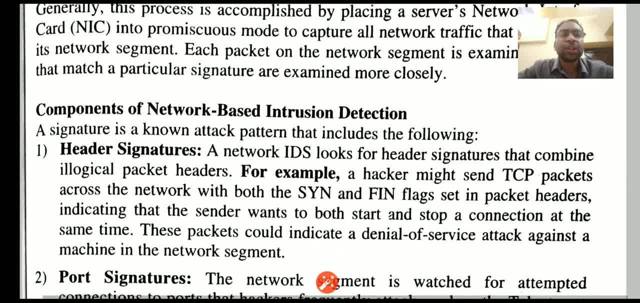 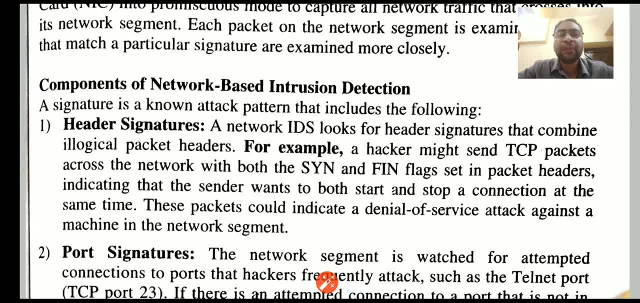 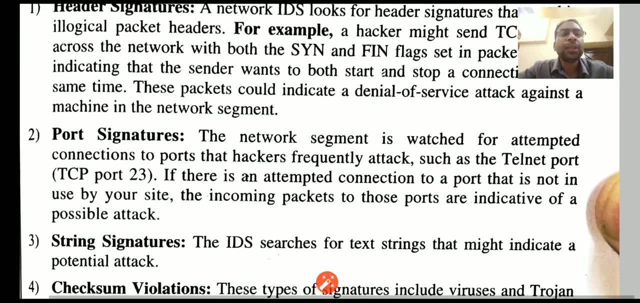 network based intrusion detection system are the header signature. They try to identify the header signature into the packet and, depending upon the header signature, they define whether the packet is a normal packet or it can be an intruder packet. They find from the recognize the port. 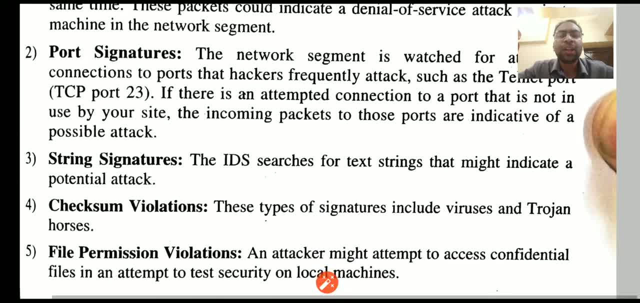 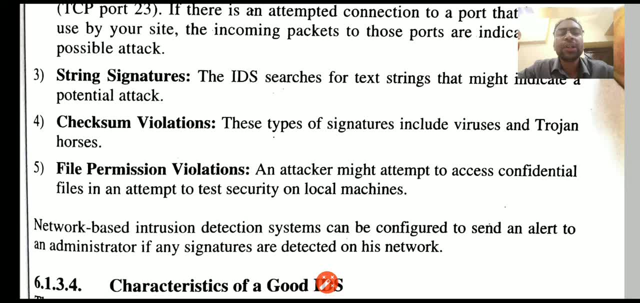 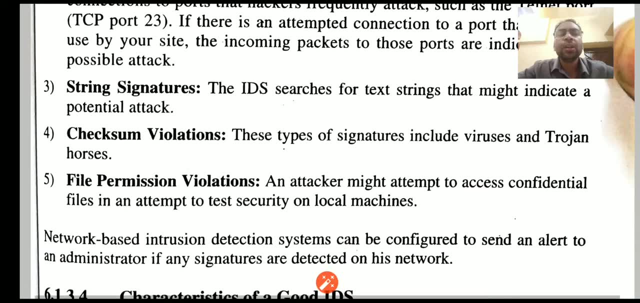 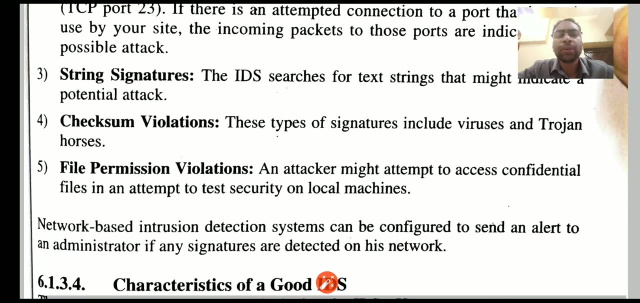 signature also, Then string signature, the checksum validation is performed. File permission validations are also performed. So these are the components and checks that are performed by the network based intrusion detection system to identify whether data or a packet is a normal packet or it can be a packet related to some. 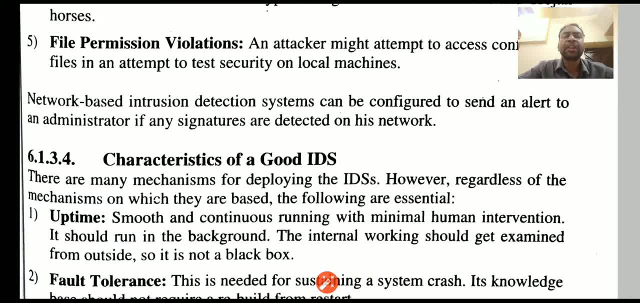 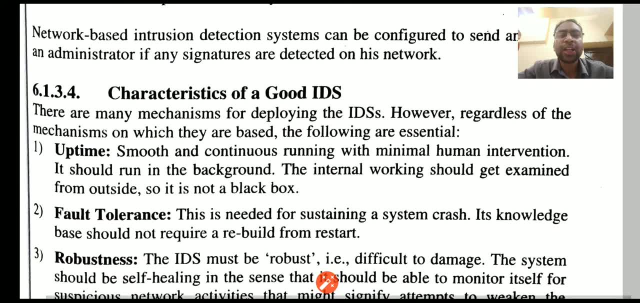 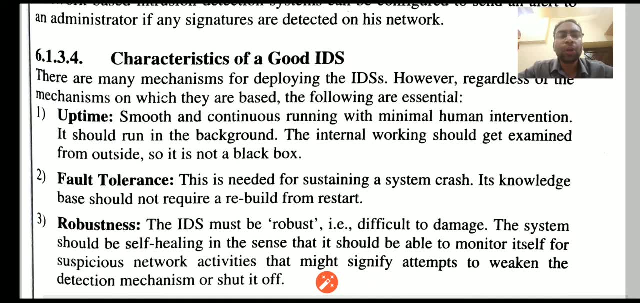 intrusion. Now let's talk about the characteristics of good IDS. So the first characteristics is a good IDS is uptime. Uptime means it should not take much time in getting initiated, getting started. Then the fault tolerance: it should be capable of tolering the faults. Robustness: it 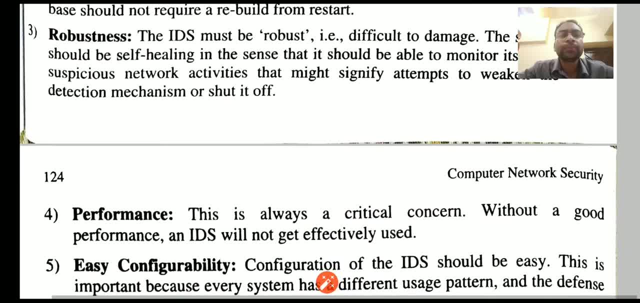 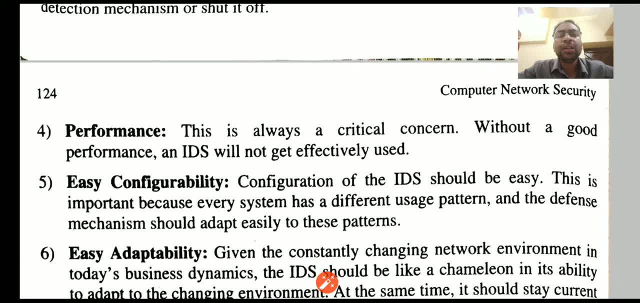 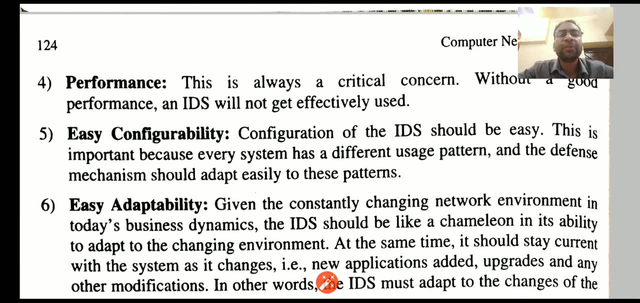 should be robust enough to perform under good or bad conditions. The performance should be good even into the critical sections. also, Easy configurability: it should be such that it can be configured configured with much ease. the configuration should not be very complex. easy adaptability. 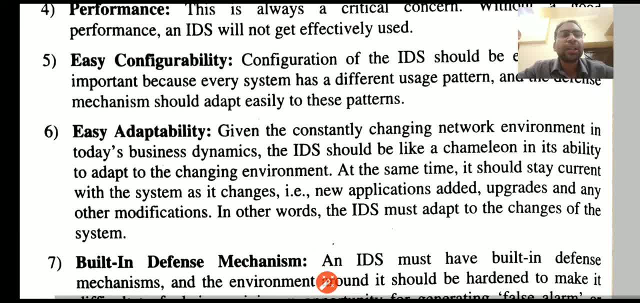 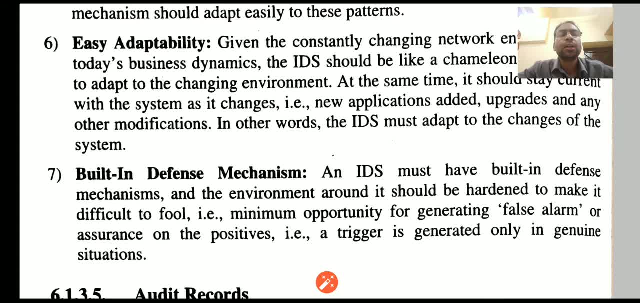 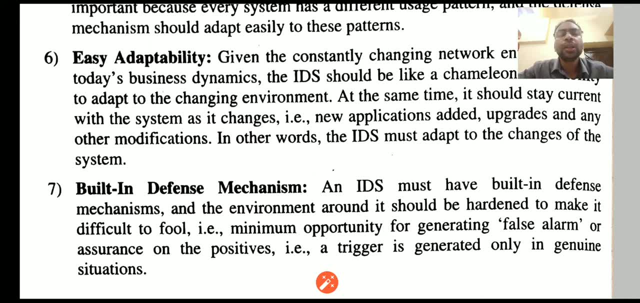 so that it can adapt to different situations, different environments and different techniques. built-in defense mechanism. it should also have some rules and policies defined into the system so that it can perform accordingly, and it it should be capable of identifying the intrusion and detection accordingly. so that's it for the lecture. you can pause the lecture. 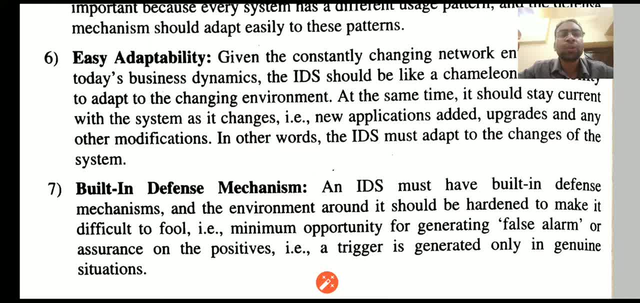 and you can refer the notes i have given. i have already given to you and for any query and any comments, feel free. thank you. 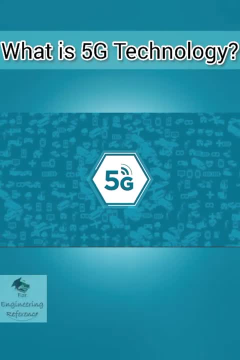 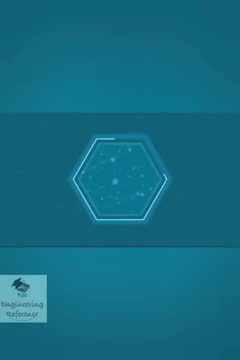 5G is the 5th generation mobile network and its speed is up to 100 times faster than 4G. It is a new global wireless standard after 1G, 2G, 3G and 4G networks. 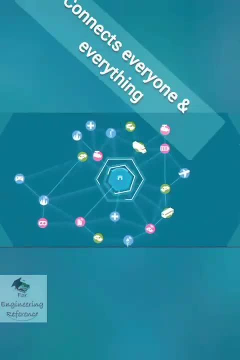 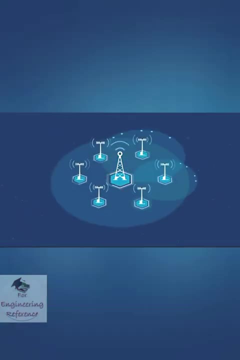 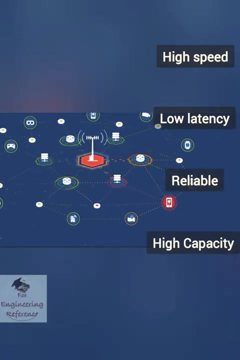 5G enables a new kind of network that is designed to connect virtually everyone and everything together, including machines, objects and devices. 5G wireless technology is meant to deliver higher, multi-gigabits per second, peak data speeds, ultra-low latency, more reliability, massive network capacity, increased availability.